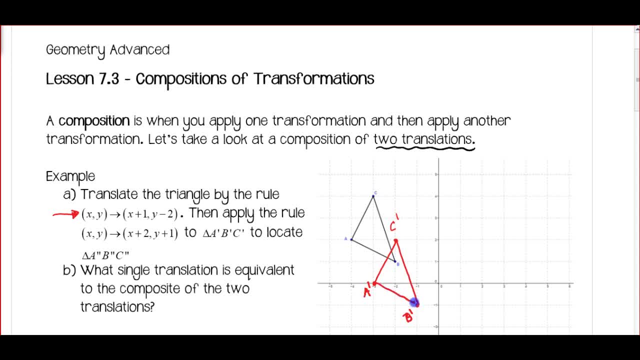 triangle And we can see that it's been translated to the right. The whole thing is right: one and down, two units. So now I'm going to take my new triangle and I'm going to apply the second transformation so that I have a composition of translations. So now what I'm going to do is I'm going to add two to each x value and add one to each y value. So let's start again with A. I'm going to add two to this one. 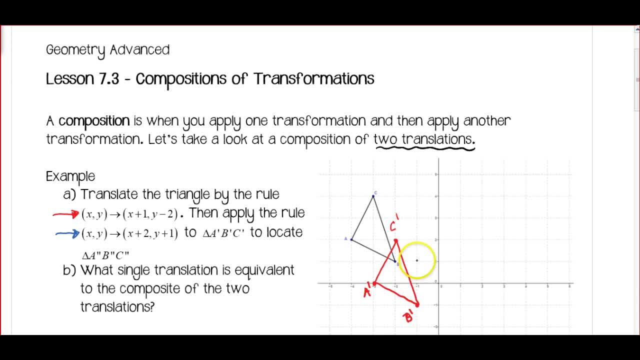 the x's. so move right two. add one to the y's, move up one. so here's my a double prime. and then for point b, to the right, two and up one. so here's my b double prime. and the same thing with c prime. i'm going to move to the right, two and up one. so here's my c double prime. finish it off by drawing. 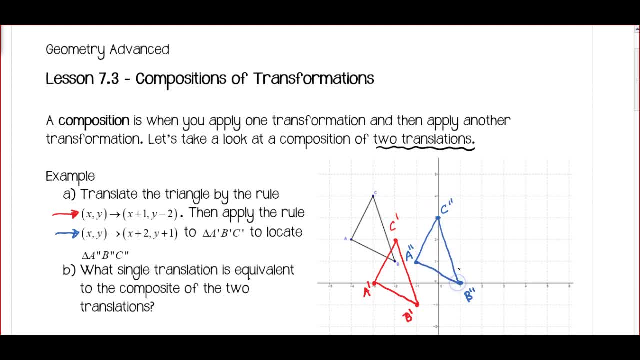 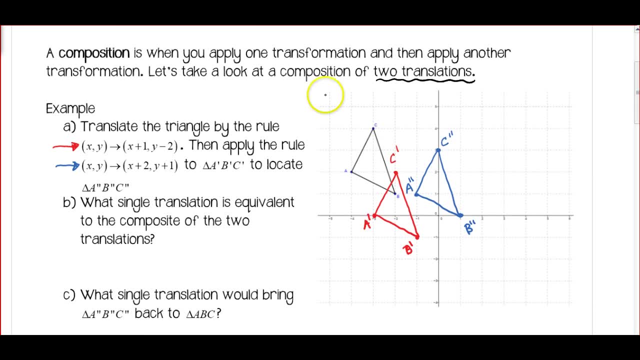 the triangle, and here's my second translation. so if we look at this picture, we could have gone directly from this first one to the third triangle. so for the first question, what single translation is equivalent to the composite of the two translations? so go ahead and if you want to, 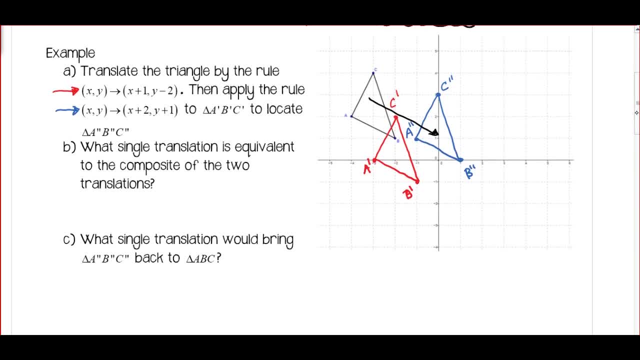 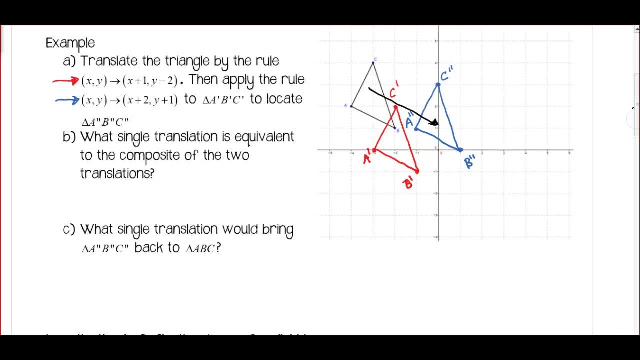 pause the video while you think about it and i'll see you in the next one. think about that and answer that. go ahead, and we'll talk about that when i see you next in class. we'll make sure we all are on the same page. and then part c: what single. 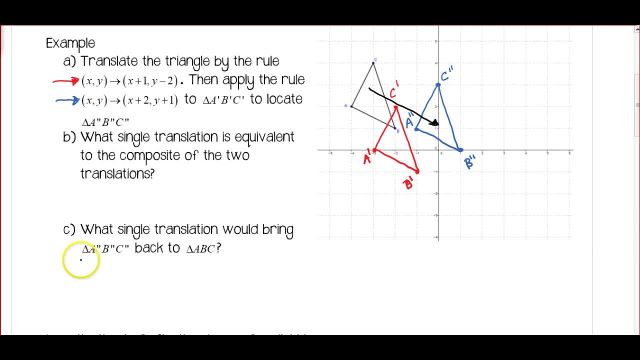 translation would bring triangle a, prime b, a, double prime b, double prime, c, double prime- back to the original triangle, so going backwards, what translation would work? so for both of these we want to rule x, comma. y translates to: and then you're going to fill it in. 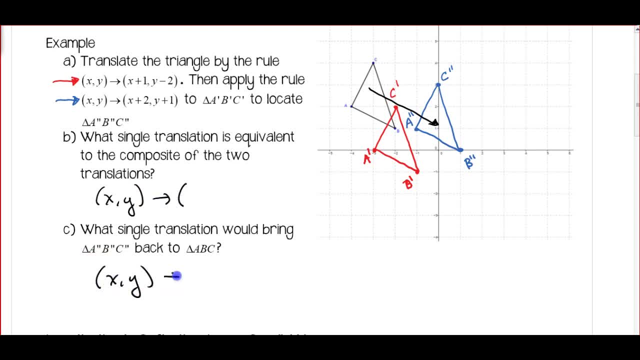 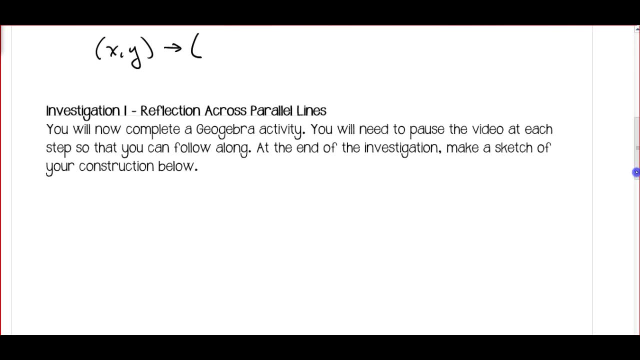 and over here we're going to fill it in, and over here we're going to fill it in, and over here we're going to fill it in, and over here x comma y, and we'll fill in that rule. now, moving on to the first investigation, which is going to lead us to one of our conjectures, we're 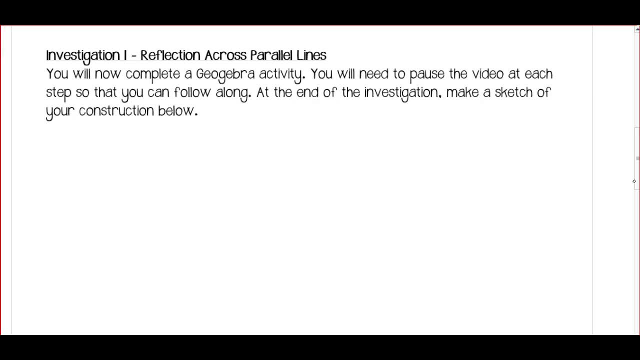 going to complete a geogebra activity, so what i want you to do is keep pausing the video and switching back and forth between the video and geogebra and do the steps as we do them. you know you can do the investigation as well. so, um, let's switch over to. 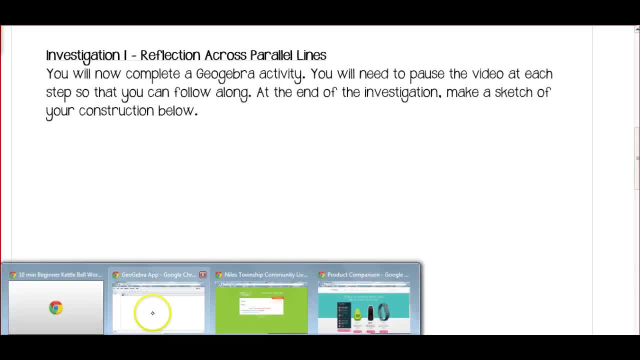 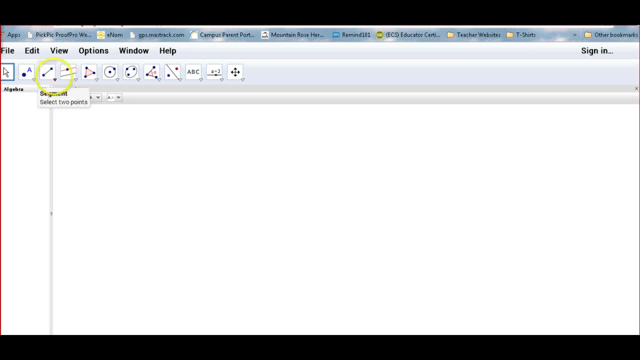 geogebra, and the first thing that we're going to do is we're going to construct two parallel lines. so let's start with a line. so i'm going to construct a line. you can construct it like i do, or you can construct it however you would like. so again, if you want to pause the video. 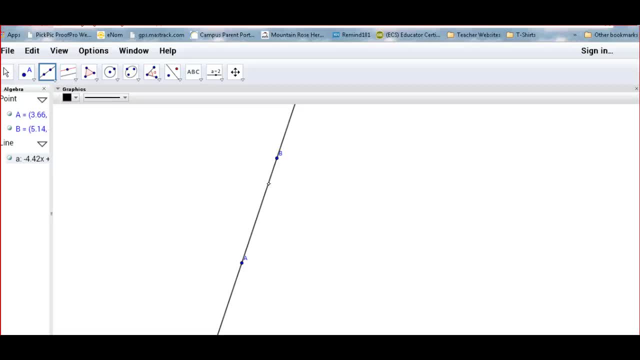 go over to geogebra on your computer and construct your line. go ahead now. what we want to do is we want to create a point. so i'm going to get my point tool up here and i'm going to create a point, and then i'm going to construct a line parallel to line a, b. 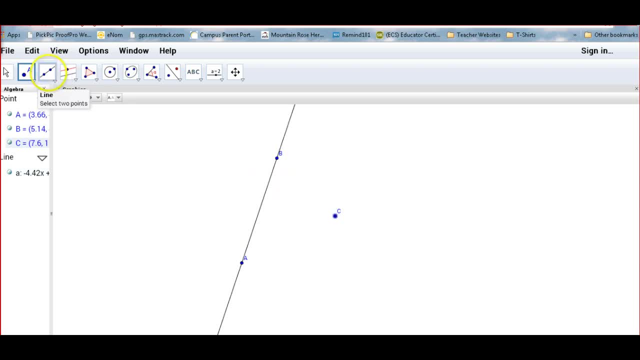 that goes through the line a b, and then i'm going to construct a line parallel to line a b through point c. so i'm going to go back here to my menus and i'm going to click parallel line. you see, the first one here is or the second one is parallel line. so make sure you have the parallel line. 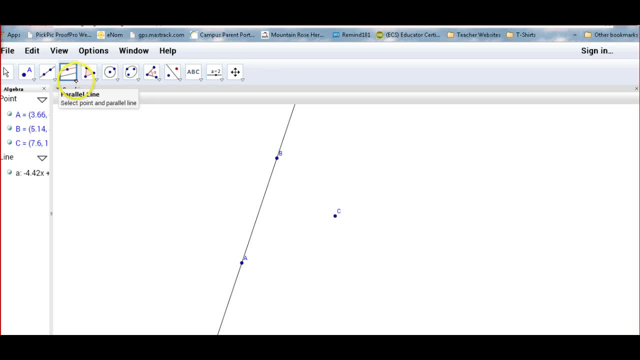 and again, if you're not sure what to do with the tool, if you scroll over that little triangle it will tell you select point and parallel line. so now i'm going to select the point and then i'm going to select the parallel line and it automatically constructs a line. 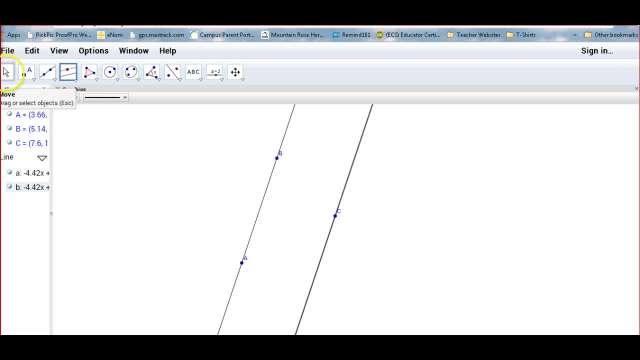 to construct this new line parallel to the first line. so if i get my cursor over here, then i move this line around. you see that my new line always stays parallel to, because that's how i constructed it, all right. so if you haven't done that, go ahead and pause the video. 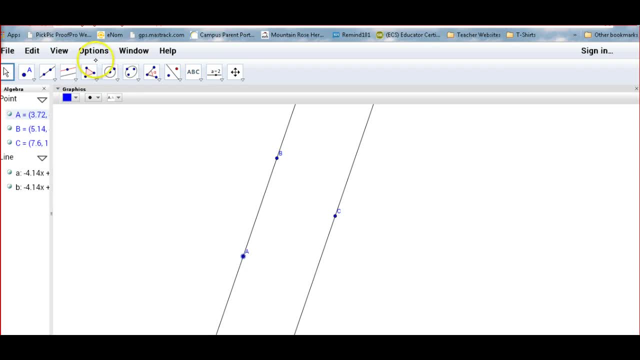 and construct your parallel line. next, what we want to do is we want to construct a polygon. so if you don't have the polygon tool, go ahead an grab that so you can draw whatever type of polygon. we want to make it so that we know where, and we're going to put it all the way on the left. so I'm just going to make some. 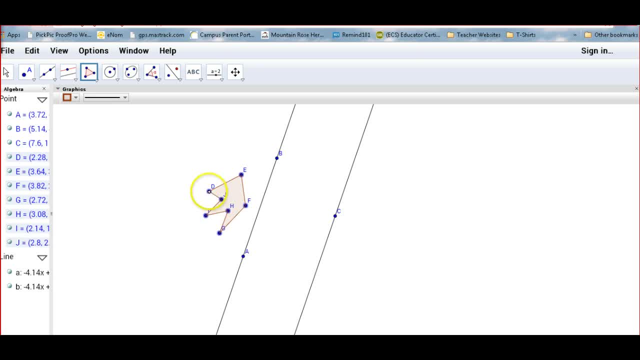 sort of a shape here. it doesn't really matter what you do. so there's my shape. and now this next menu that we're going to use. this is our transformation menu, so we're going to do the first one: reflect about a line. so you want to? 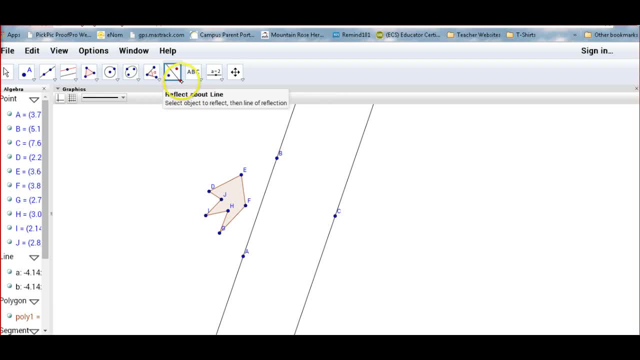 select that one and then again, if you hover over the triangle it says select object to reflect, then line of reflection. so if you hover over your polygon it will give you a pop-up that says polygon, poly one or whatever yours is. you want to click on that because if you hover over one of the other points, 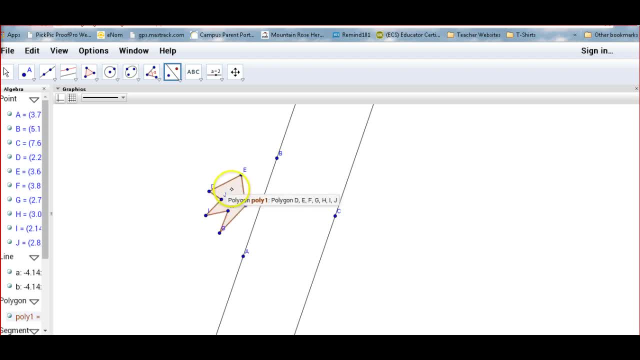 it'll say point E or it'll give you a segment. so make sure you're over the polygon and click on the polygon, and then you're gonna click on the first line and you see how it reflected it right over. so now we have a mirror image, all right. so make sure you can do that. pause your video and rewind as. 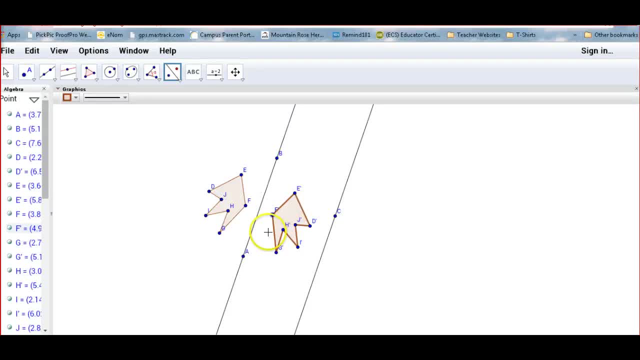 necessary to follow along with the steps. now, what we're going to do is we're going to take our new polygon, so we're doing a composition of reflections. now we're going to take this new polygon and we're going to reflect it over the next line so you can see how it's already selected here, because it's kind of 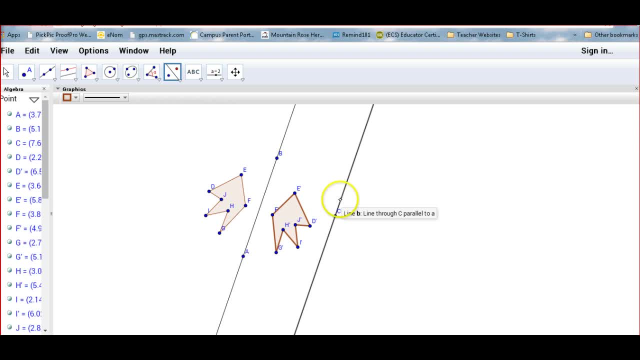 highlighted. if we click this line, hopefully it will reflect it again. well, let's try it. so let's click our menu here, select our polygon and then select our line. sometimes it takes a minute to come on. now let's try selecting our menu item again. reflect about a line, select the polygon. 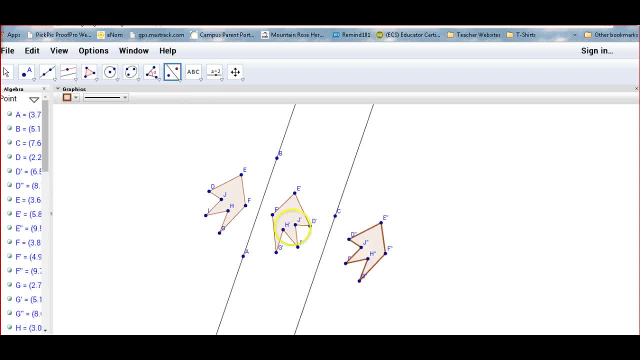 select the line. there we go. okay, so now we've got it reflected over the second line, and once you get this done, what I want you to do is I want you to draw a little sketch, in the space that I provided you in notes, of what you have here, so go. 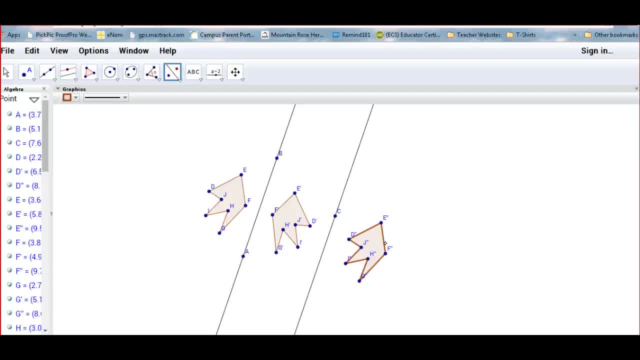 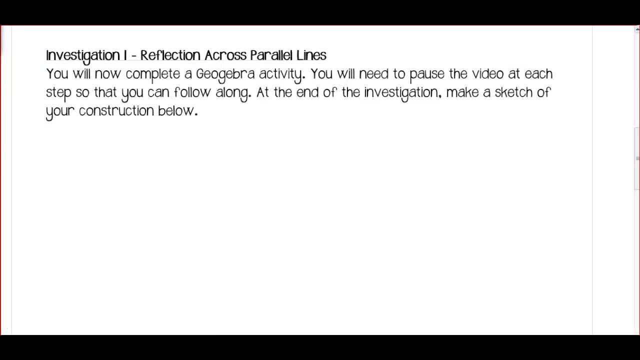 ahead and pause the video and draw on your sketch. so I'm going to go back to my notes here. so in this space you want to draw a little sketch of yours. so here's my parallel lines, and I had something like This. I'm just going to sketch it in real quick and then it looks something like this: 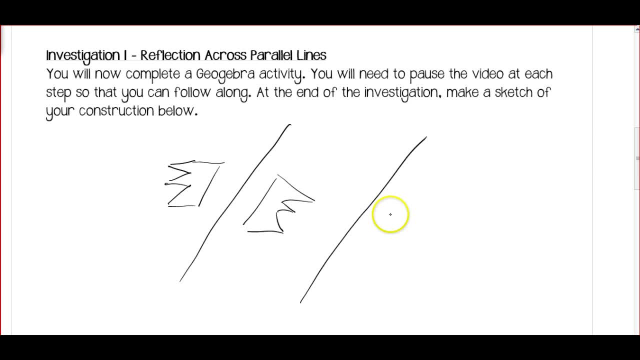 It doesn't have to be too accurate, just get it in there mostly, and then again something like this: So we sketched it in, and what I want you to do is I want you to try and figure out, if I reflect over two parallel lines, what single transformation could accomplish going. 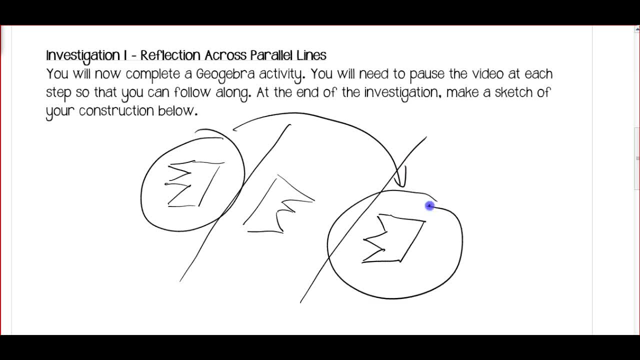 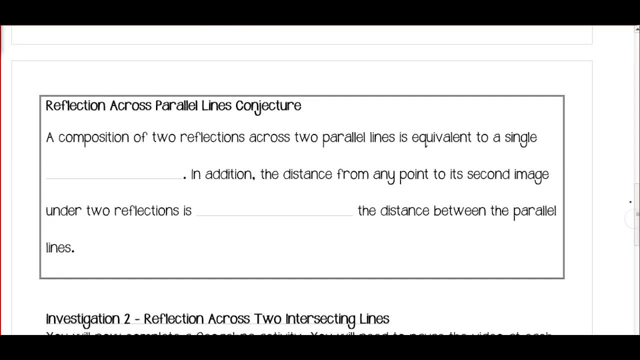 from this to this, and that's where you're going to fill out the blank lines here. If you think you know what goes there, a composition of two reflections across two parallel lines is equivalent to a single fill in the blank. we'll talk about that in class. 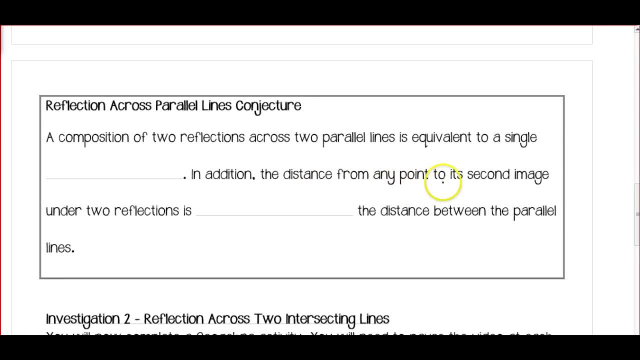 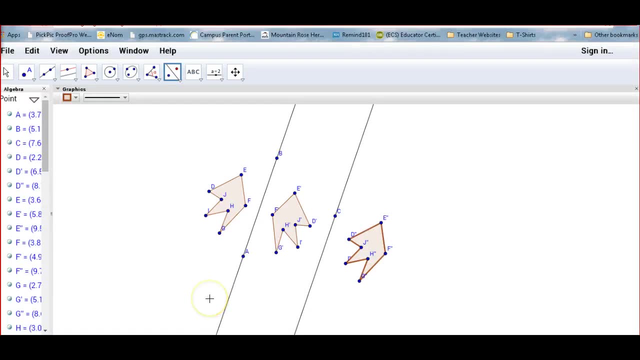 In addition, the distance from any point to its second image under two reflections is blank, the distance between the parallel lines. So if we go back to this, there's another menu over here where we can measure distances and angles. So distance or length, if you want to measure. if I want to measure the distance between: 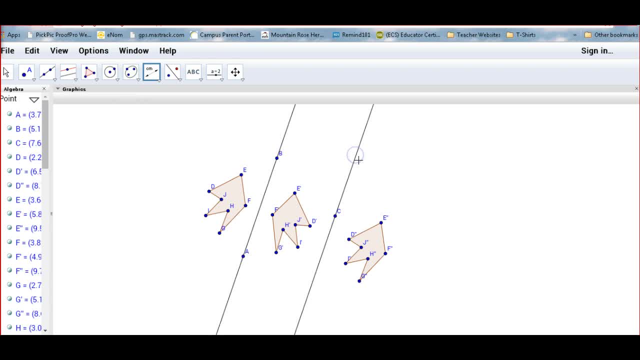 these two lines. I can just click the two lines. Let's try that again. So let's do this line and let's try the point. and what do we get up here? Hey, that's not what I wanted. All right, let's try that one more time. 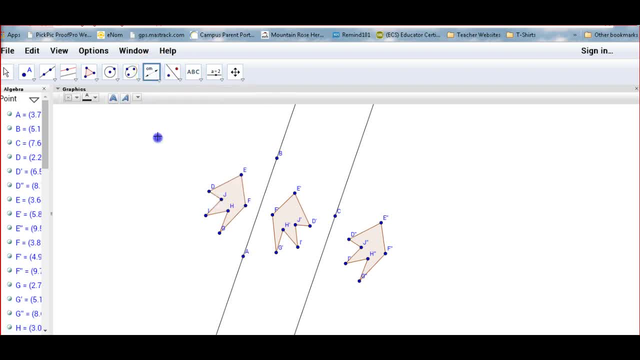 Let's select our menu here and we've got distance or length, so I'm going to select this line And I'm going to select this other point that should give me the distance. yep, there we go. So the distance between this line and this point is 3.12.. 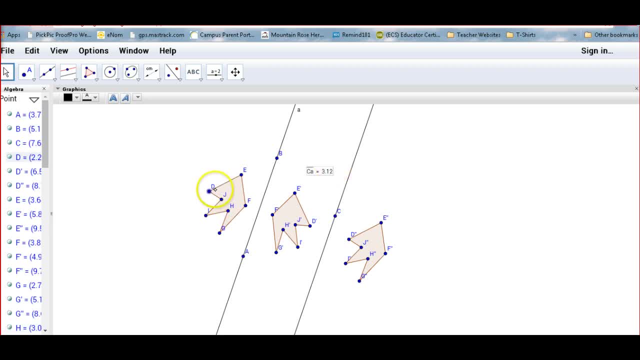 So then, what you can do is pick any point on the original image and any corresponding point on the second image and find the distance between those And see how it relates to, And let's do this distance here. so that's what you're going to do on your own. 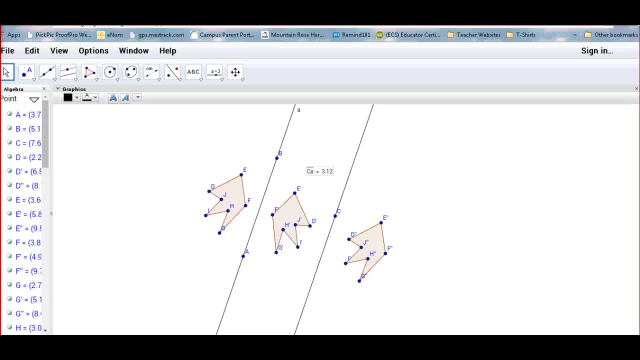 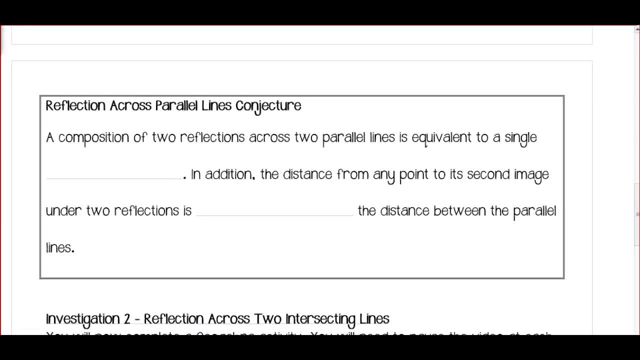 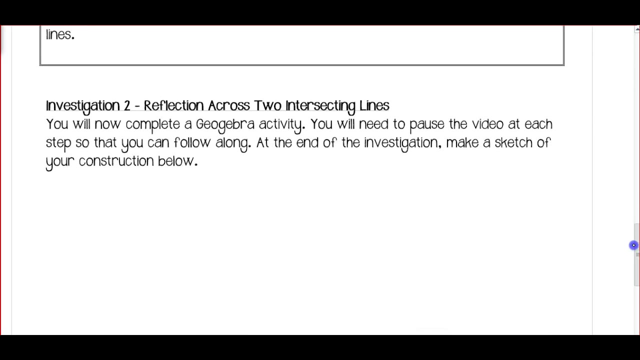 So go ahead and pause the video and work on what you need to, and then we'll go back to the notes. All right, so do your best at filling out the blank lines on that. conjecture Investigation 2,. now we're going to do a reflection across two intersecting lines. 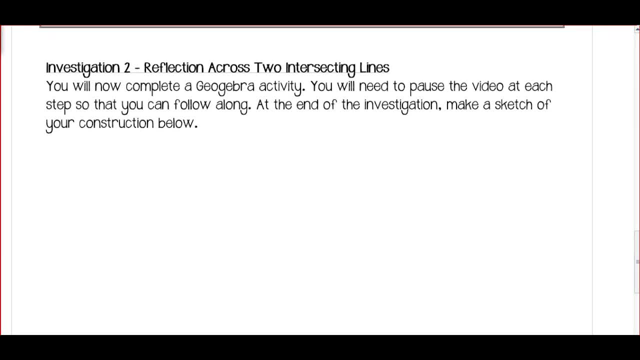 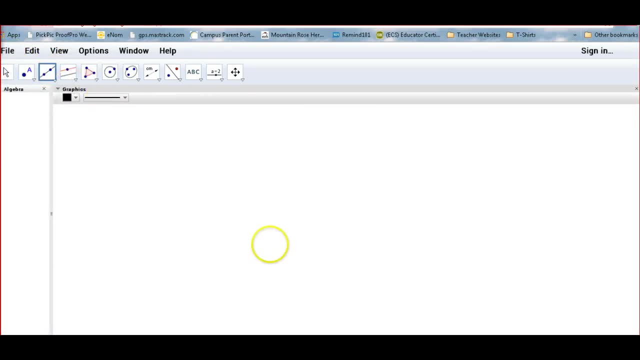 So again, pause, as you need to to follow along. So we're going to go back to GD2.. All right, GeoDriver, here I'm going to make a new file and I'm going to draw a line, And then I'm going to draw another line that intersects this one. So I'm just going to go. 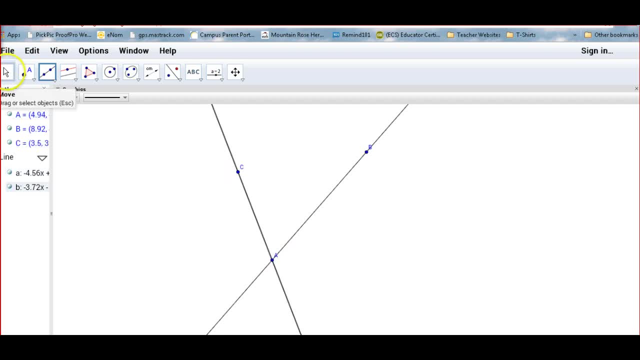 through point A. So now I have two intersecting lines. I could change the angle between them as I want to by dragging either one of these. All right, again, pause when you need to. Now I'm going to construct a polygon all the way over. here. on the left I'm just going to make a quadrilateral. 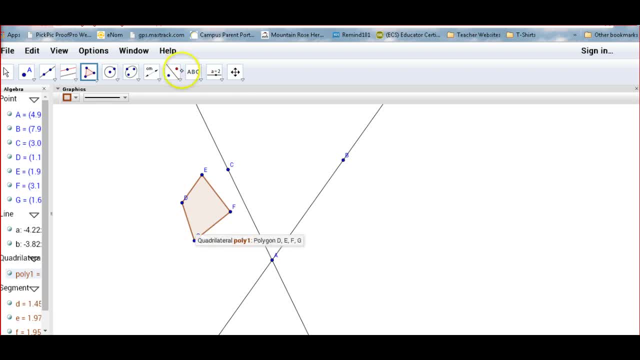 here And once you have your quadrilateral, we're going to go back to our transformation menu. We're going to reflect about a line. So remember it's select object to reflect, then line of reflection. So I'm going to select my quadrilateral and then I'm going to select my line. Try that again. 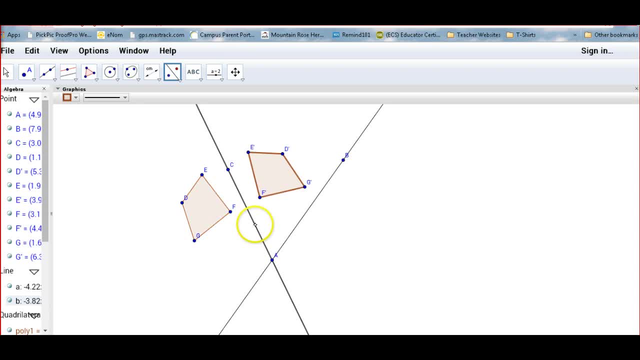 So I'll select that, Select that. There we go, All right, so go ahead and do that. Pause if you need to, And then I'm going to reflect this image over the next line. So select my menu again. Select my polygon. 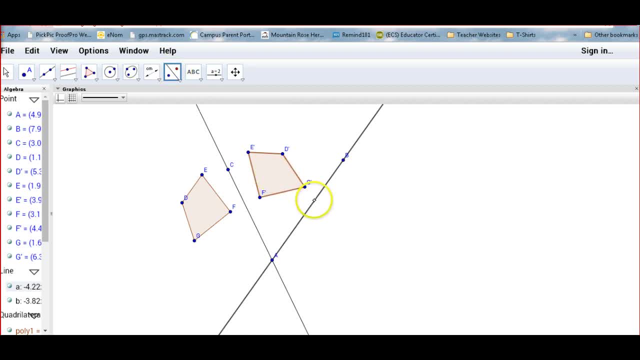 Select my line. The stylus is a little tricky. There we go. Okay, so here's my second image. So now we can see that this one is a reflection of that one and the second one is a reflection of the first one. But I want to see: how does this first image relate to this second image?